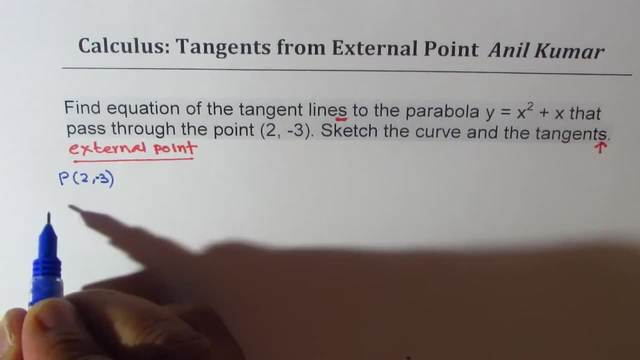 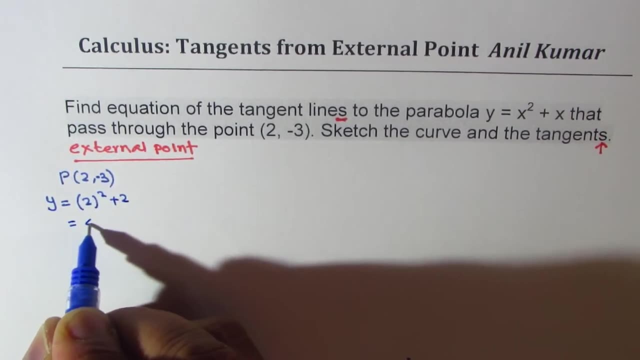 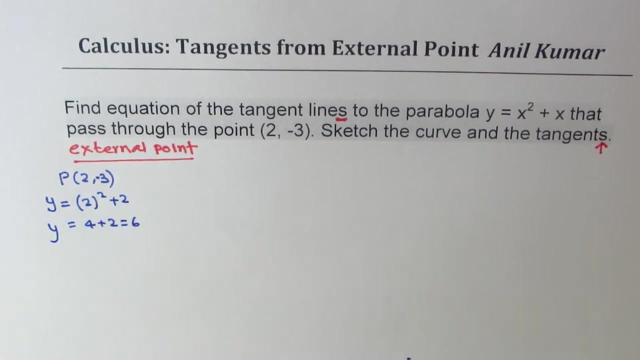 If I substitute 2 for x, what do I get? So what is y equals to? If I substitute 2, I get 2 square plus 2, which is 4 plus 2, which is 6.. So the value of y is 6 and not minus 3.. So therefore, the point 2 minus 3 is an external point. 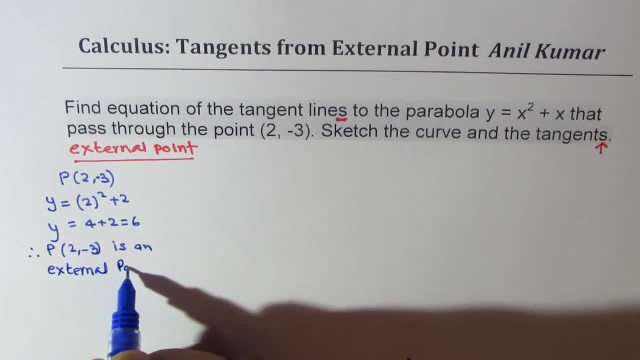 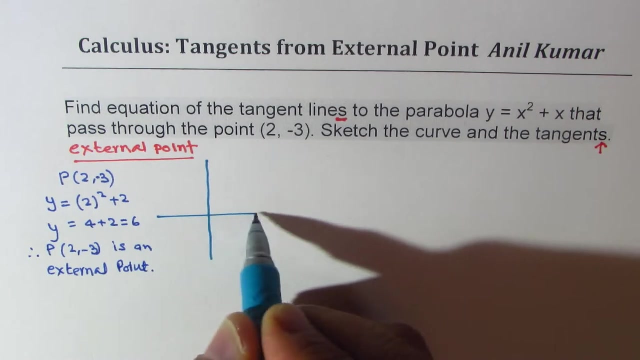 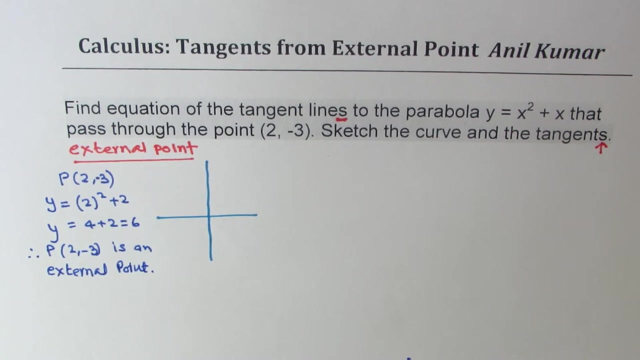 So you get the idea. So what I am trying to say here is that in our given scenario, if we have a parabola which is given by this equation, the x intercepts being clearly at 0 and minus 1, right? 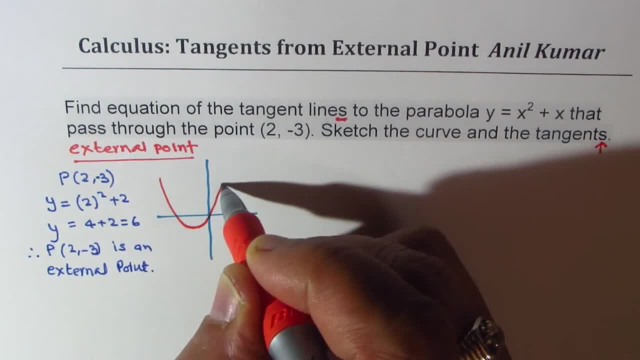 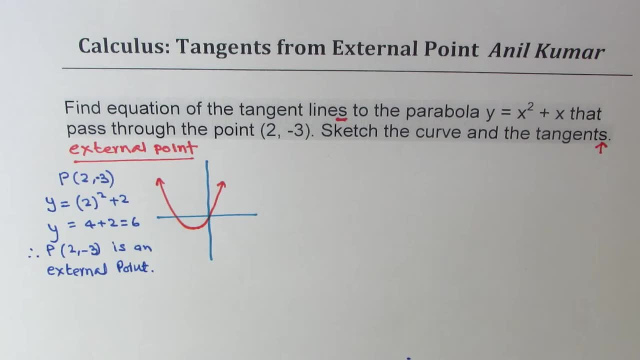 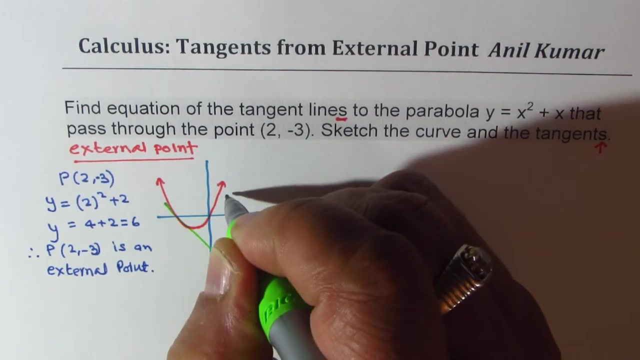 So the parabola will be kind of like this: In that case, the point given to us, which is 2 minus 3, is somewhere here. It's somewhere here. So we are looking for a tangent Which will be kind of like this: You understand, We are given a point here. 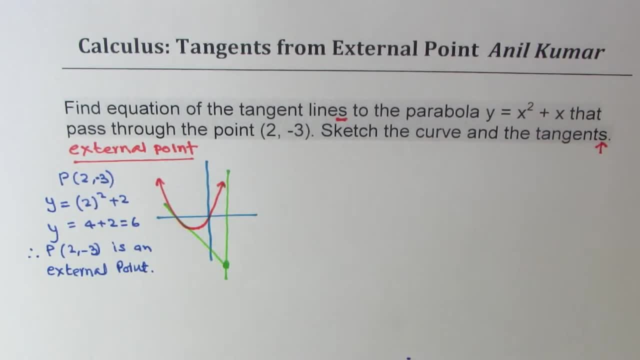 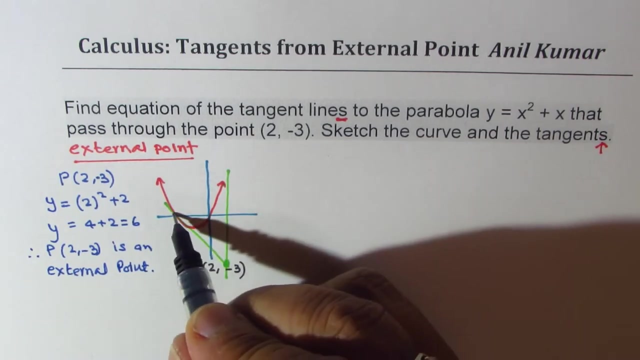 So we have two tangents. So I hope this point is very clear. So what we are given here is a point P which is 2 minus 3.. So it is an external point. So we really don't know where on this curve we are going to get the tangent. 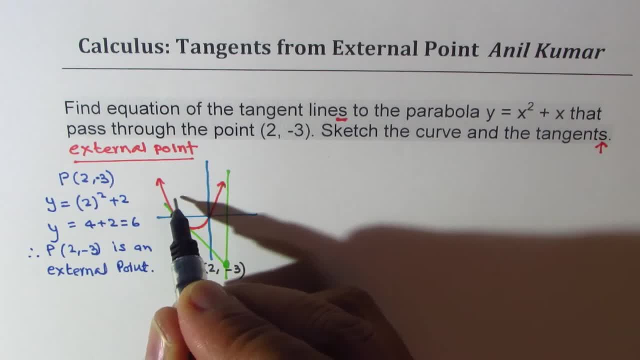 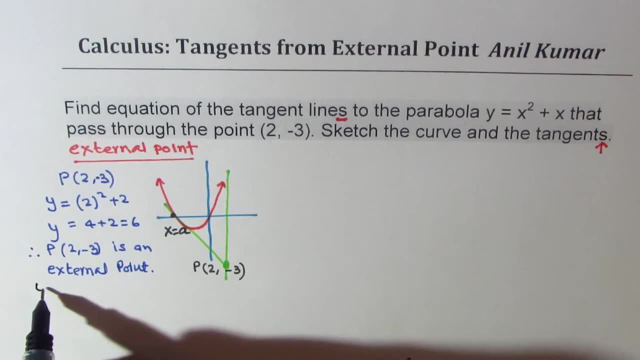 So what we will do here is to assume This point 2B at x equals to A right. So what we are saying here is: let point on the curve B. if x value is A, then the y value will be A square plus A. 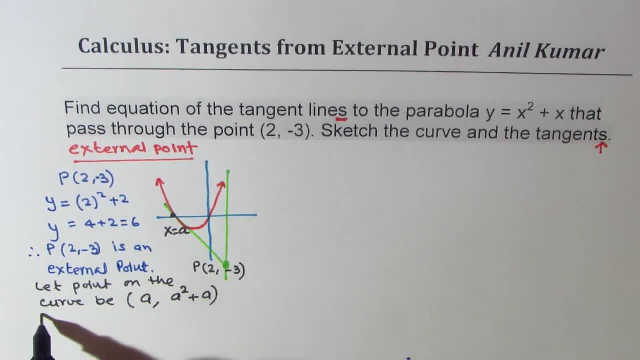 You get the idea right. Since the equation is y equals 2.. Since y equals 2. So x square plus x, You get this part right. So this is a very important part to understand before even we begin our solution, correct. 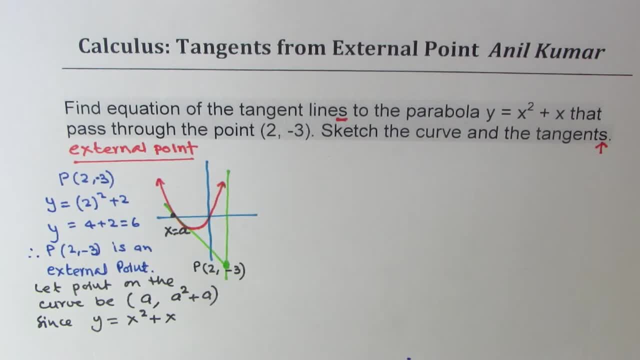 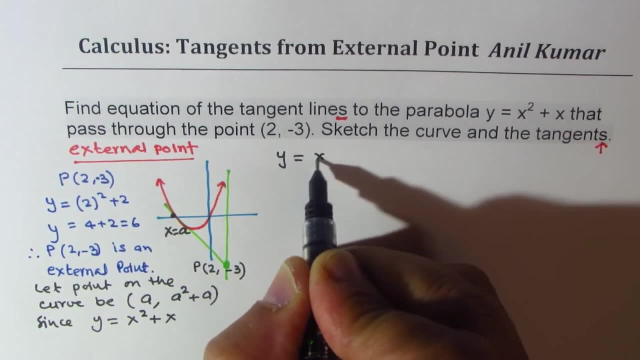 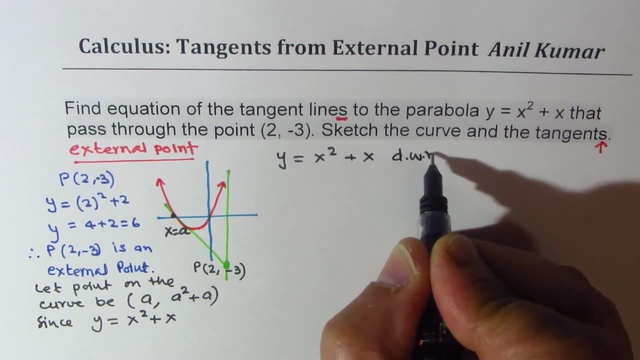 Now let's look into our solution and see how to find the solution. Okay, So we could find slope of this equation, which is y equals to x square plus x, by finding derivative. So, if I differentiate with respect to x, 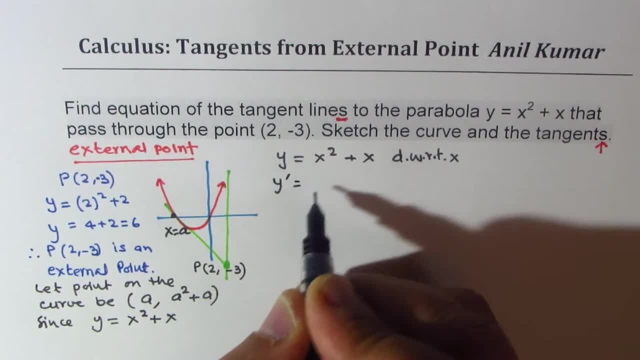 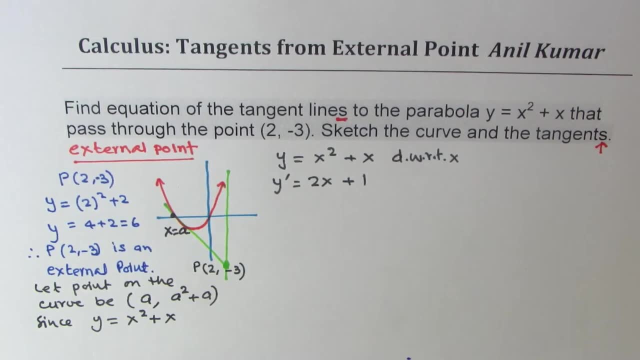 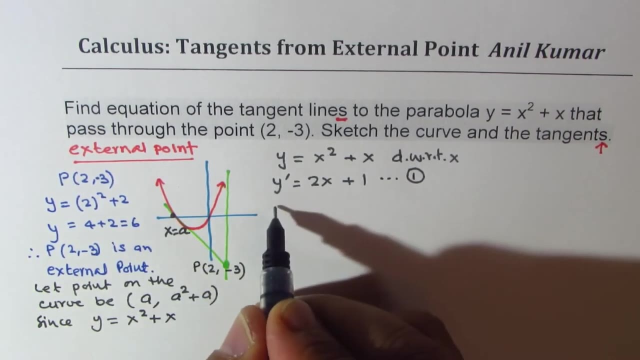 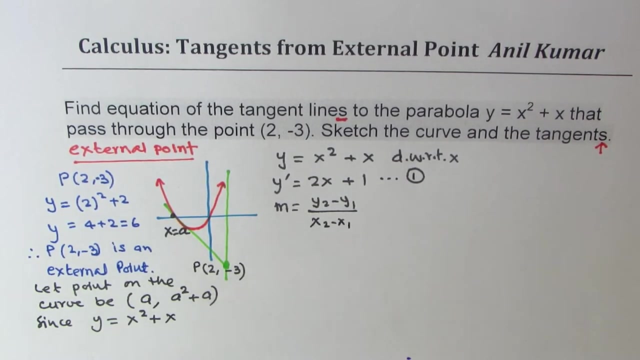 I get dy dx. Let me write: y dash equals to 2x plus 1.. So that's the derivative. We'll call this as our equation number 1.. We could also find derivative using slope intercept. So we can say: y2 minus y1 divided by x2 minus x1 is also slope. 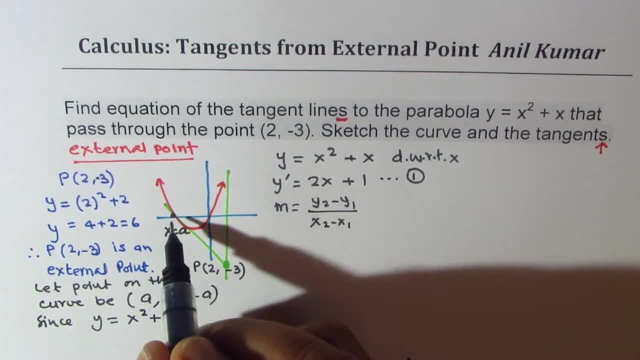 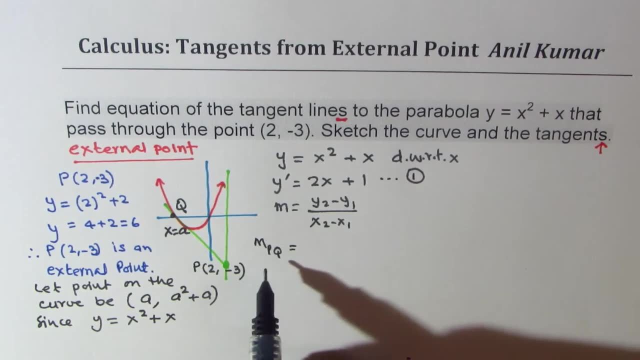 So we have two points, One point P And let this be The point Q. So the slope between the point P and Q will be: y values are a square plus a minus 3.. So that is plus 3 divided by the x values: a minus 2.. 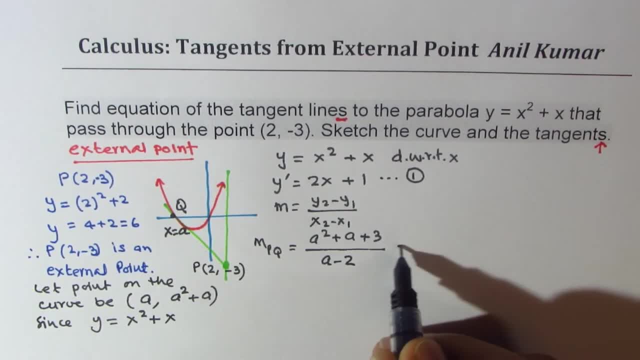 a minus 2.. So that becomes the slope And this slope we are saying equation 2.. Now, since this is a slope, This is a general slope. So from equation 1 at x equals to a, the slope is going to be 2a plus 1.. 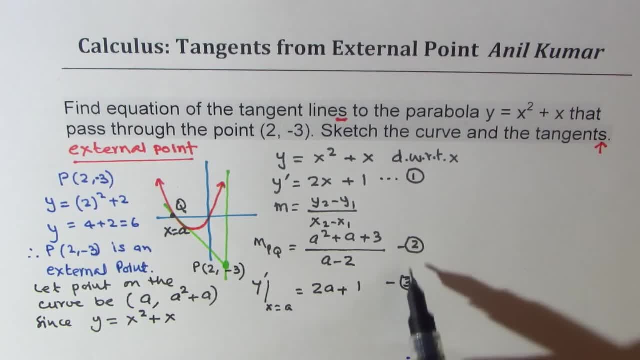 Correct, Let's call this equation 3.. So these two equations should be same, Right, Since the slope is same. So what we have here is that the m is equal to y, dash at x equals to 2.. So the slope is going to be: y dash at x equals to 2a. 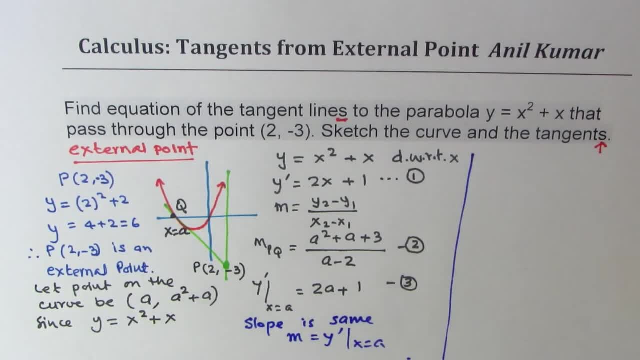 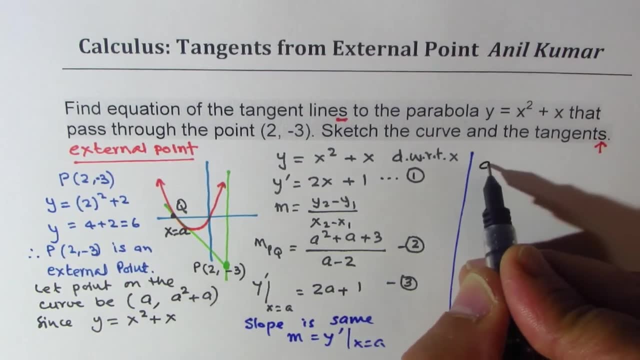 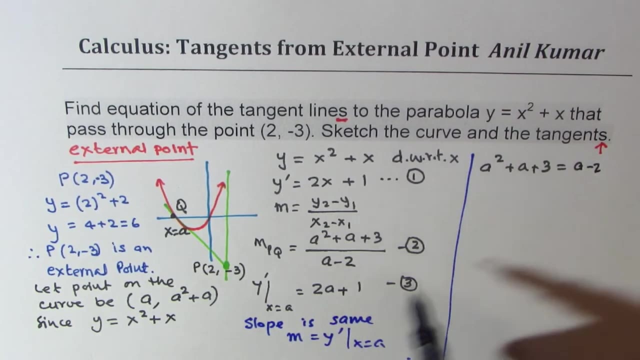 Right, So with that condition we can find what point a is. So we will now equate 3 and 2.. So we get a square plus a plus 3 equals to a minus 2.. I mean well, just okay, let me write like this: 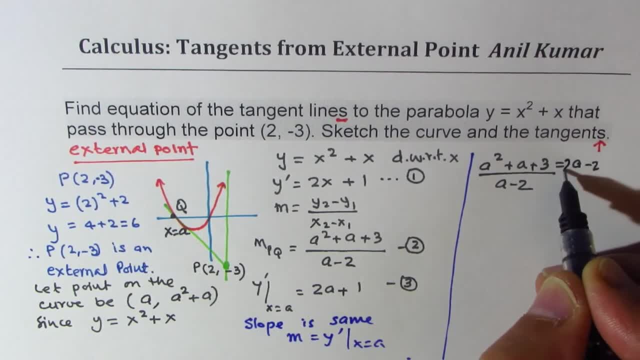 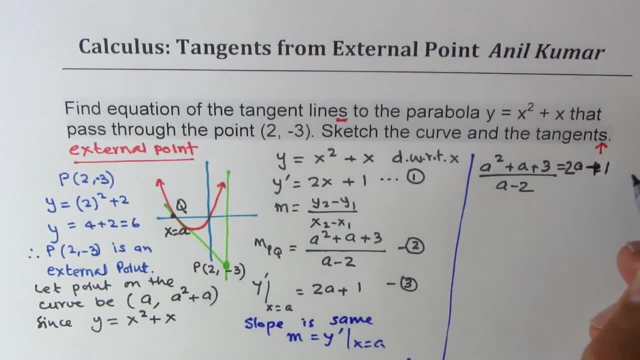 Right. So we are saying we are equating: equation 2 equals to equation 3.. This is what we are doing Now to solve it. let's cross, multiply So we get a square plus a plus 3 equals to a minus 2 times 2a plus 1.. 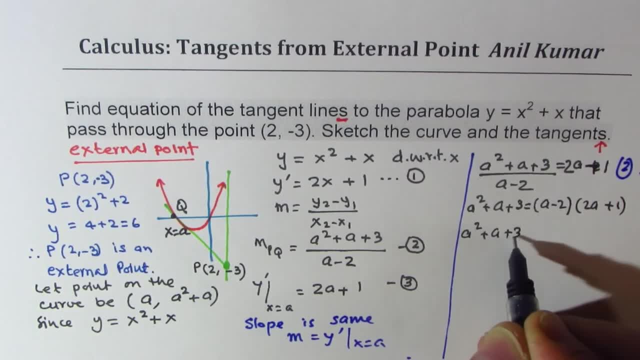 Let's expand a square plus a plus 3 equals to: when you expand this, you get 2a square Right, So you get a square plus a minus 4a minus 2.. Now bring all the terms together to find a. 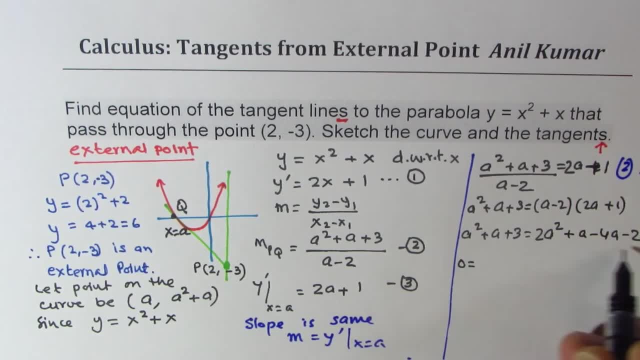 So we have 0 equals. let's bring all the terms to the right side. So 2a square minus a square. then we have plus a minus 4a. We'll take away this a and then we have minus 2, minus 3.. 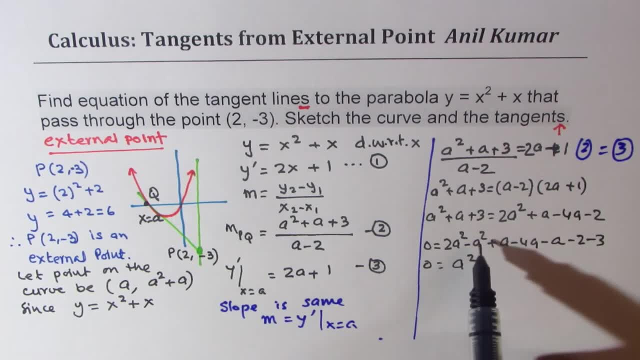 Right, So we have 0 equals 2.. 2a square minus a square is a square. Then we have a minus 4a minus a gives us minus 4a. Minus 2 minus 3 is minus 5.. 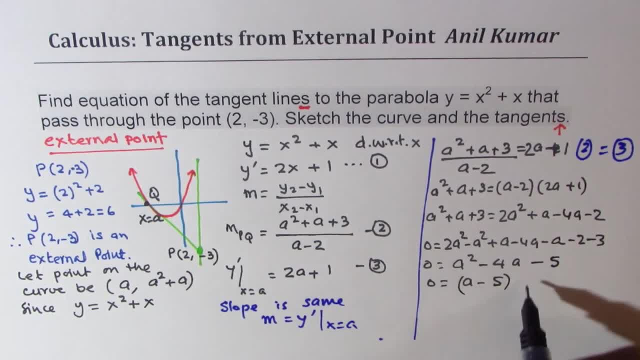 This could be factored a minus 5 times a plus 1.. So that gives you two solutions: that a could be equal to 5 or a equals to minus 1.. Correct, So we have two points where a could be equal to minus 1.. 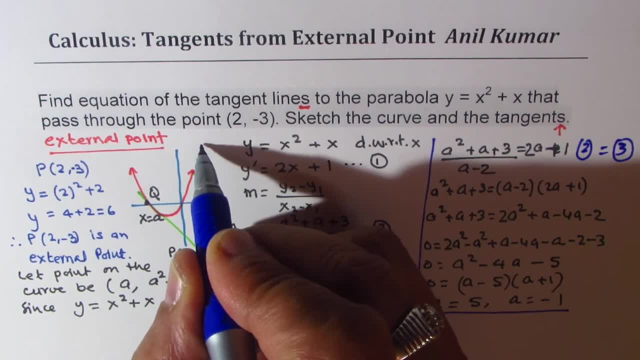 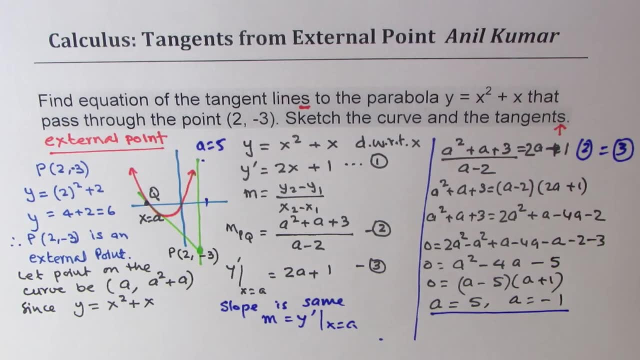 So let's say this is a minus 1. Over there we'll have a equals to 5. That means the x value, Is that okay? So we have two points. Now let's find the equation of these two tangents. 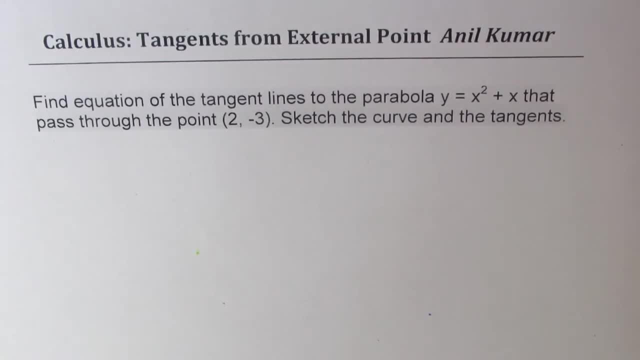 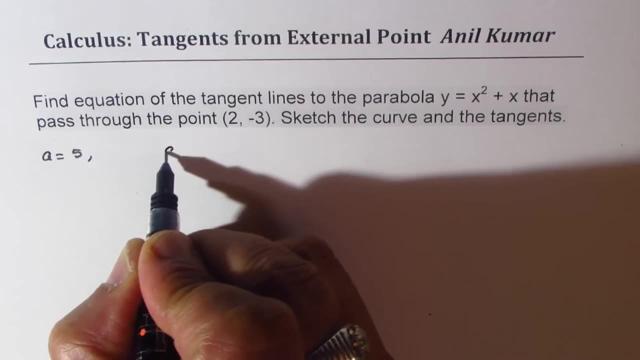 Now we'll take it to the next page with a equals to 5 and minus 1.. So we have two points. One is for a equals to 5 and the other one a equals to minus 1.. So the equation is y equals to x. 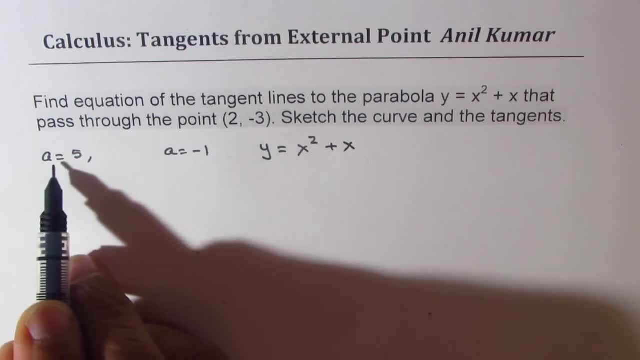 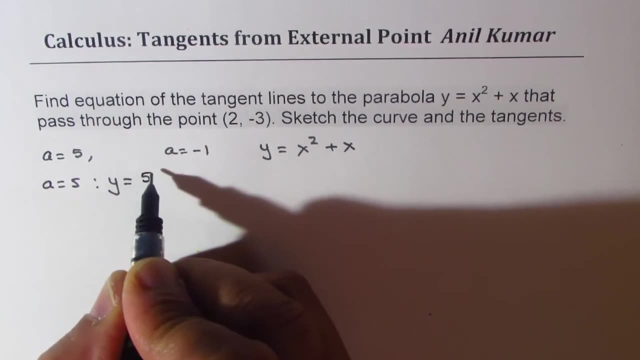 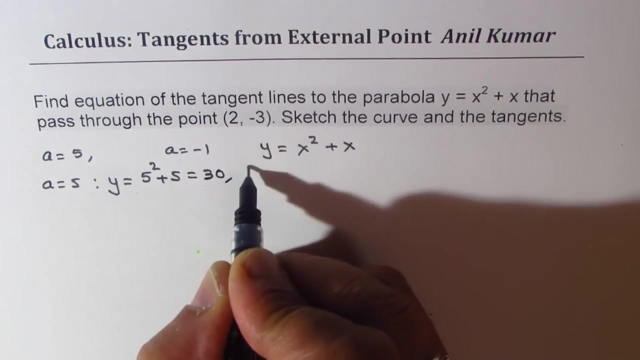 So if I substitute a equals to 5, what do I get? So if I substitute a equals to 5, I get y equals to 5 square plus 5, which is 25 plus 5 is 30. So the coordinate points are 5 and 30.. 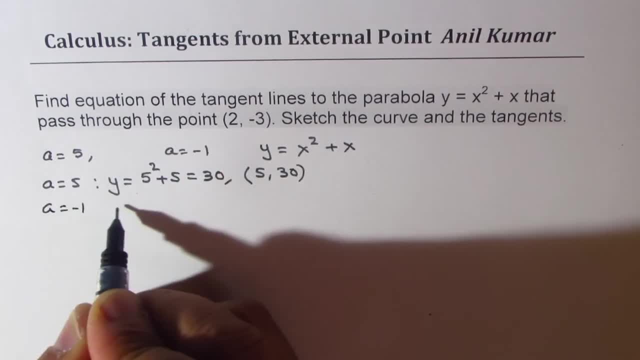 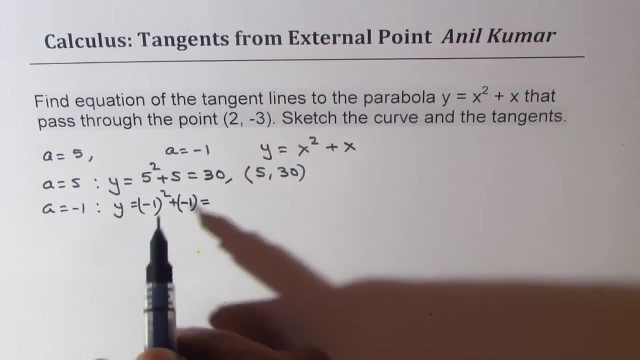 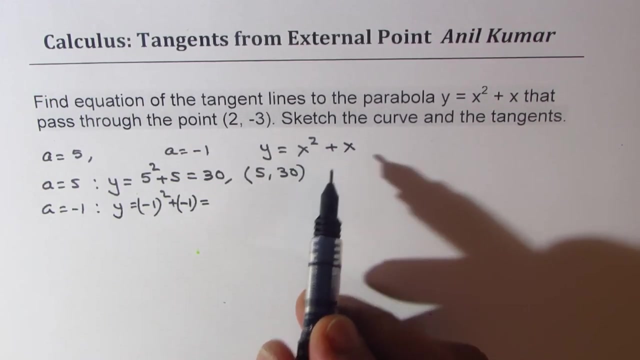 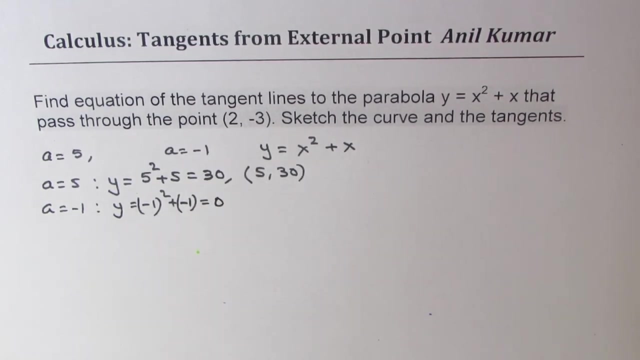 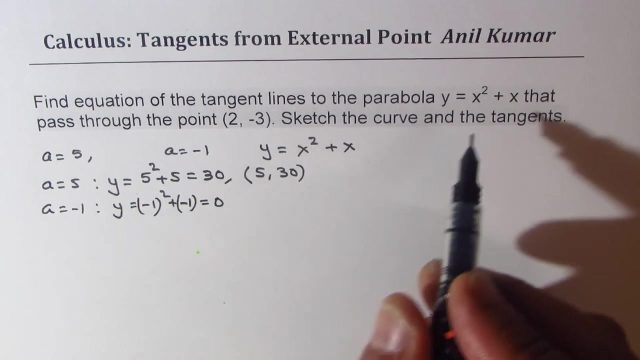 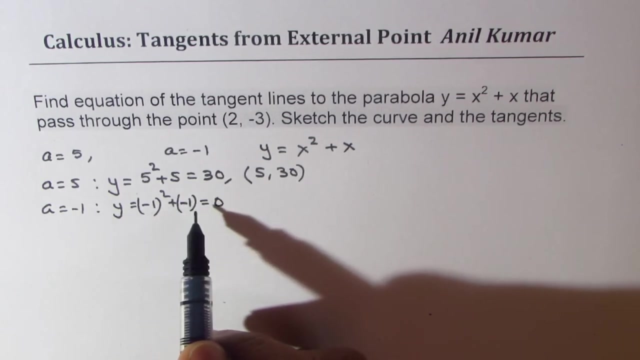 If I substitute minus 1, then I get the y value as minus 1 square plus minus 1.. Which is so, for minus 1 square is positive 1 and x means minus 1, I get 0.. So in that case my coordinate point at minus 1 is the y intercept. 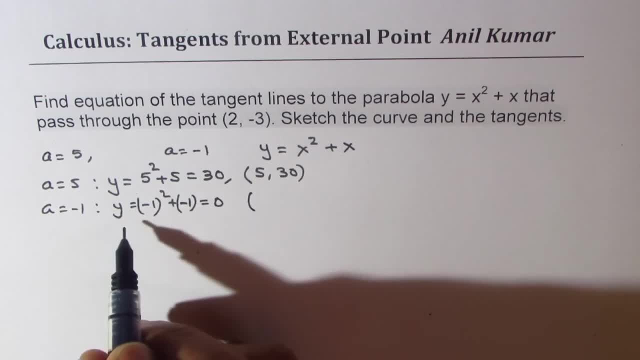 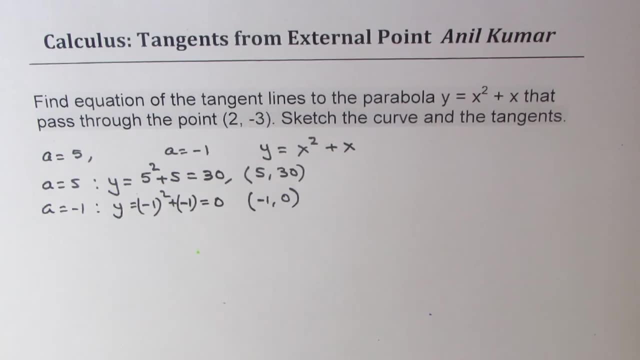 So in that case my coordinate point at minus 1 is the y intercept, So the point here is basically equal to minus 1, 0.. So these are my two points. Now what we need to do is to find equation of tangent lines. 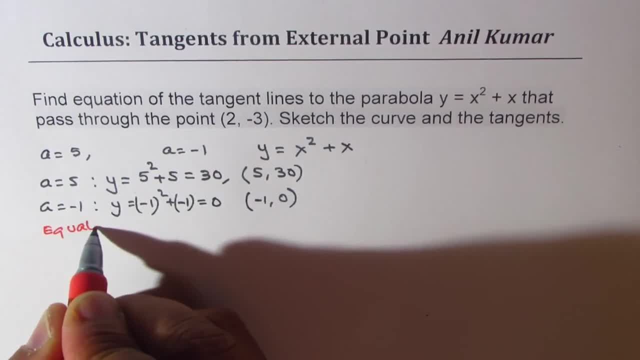 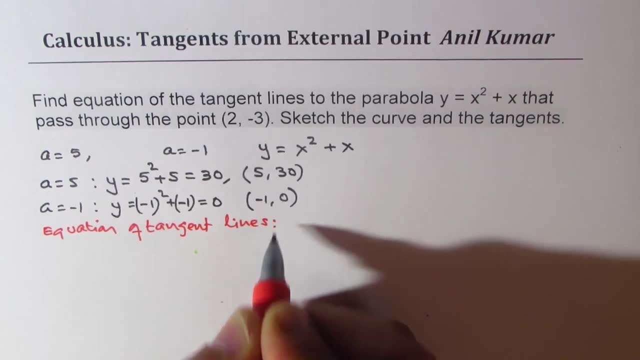 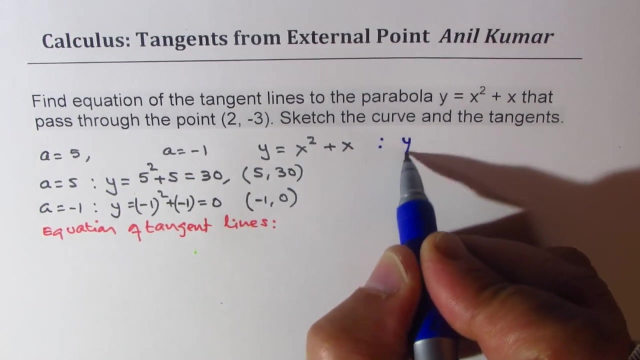 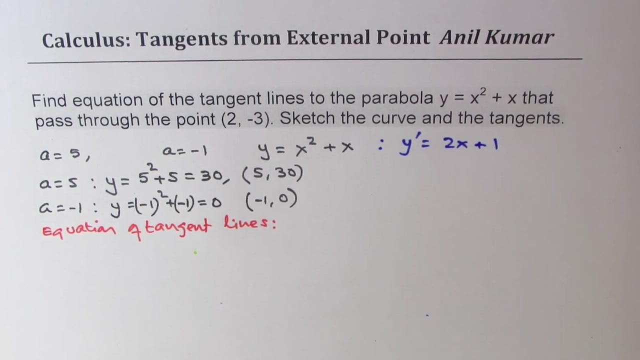 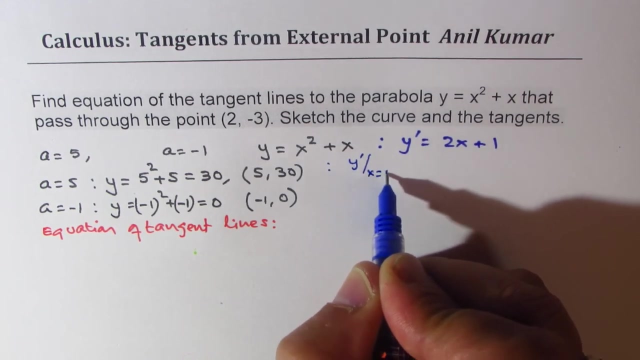 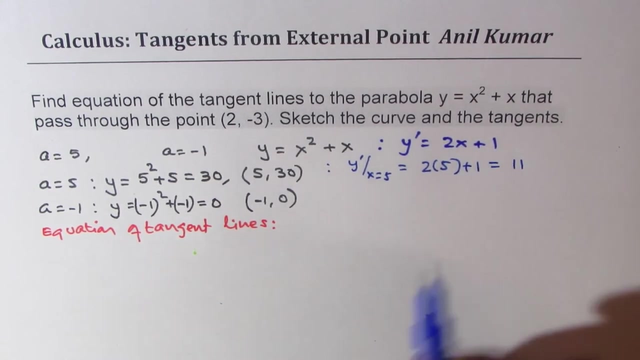 So now let's find equation of tangent lines. Well, we also know that for the equation, this, the slope is basically 2x plus 1, correct? So for these points let us also calculate these slopes. So slope y dash for x equals to 5 is equals to. let's write 5 here 2 times 5 plus 1, which is 11.. 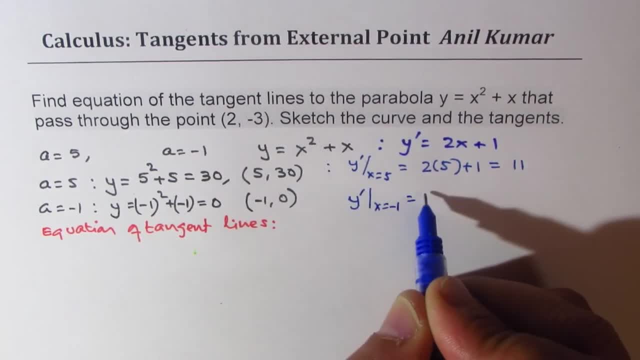 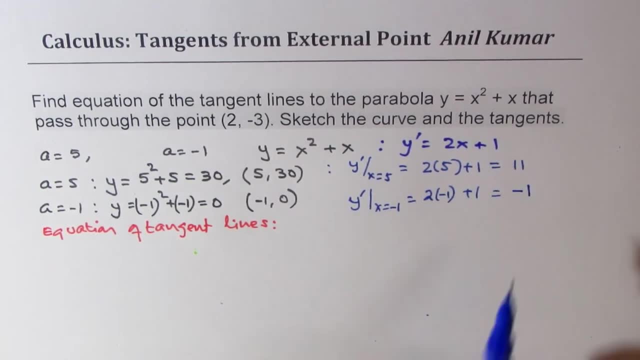 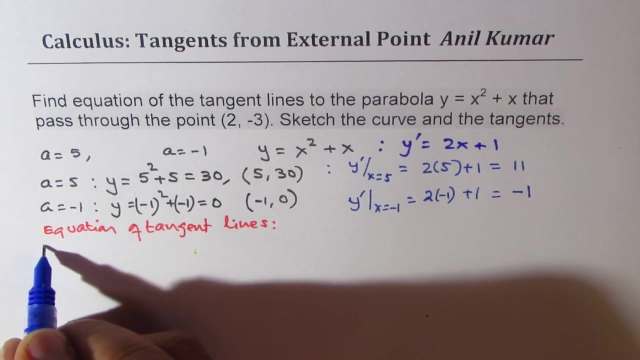 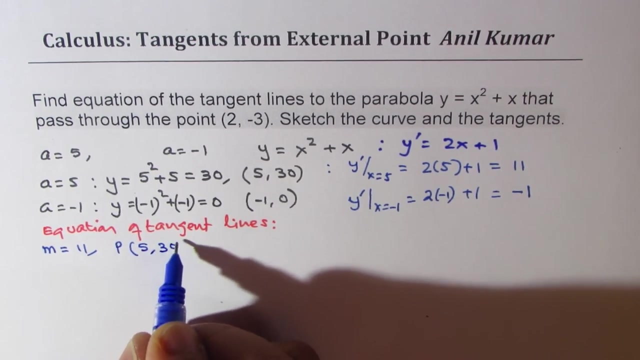 And the slope for x equals to minus 1, will be 2 times minus 1 plus 1, which is minus 1, right, So these are the two slopes. Now we can find equation of tangent lines. So let's take the line which has slope of 11 and the point being 5 and 30, good, 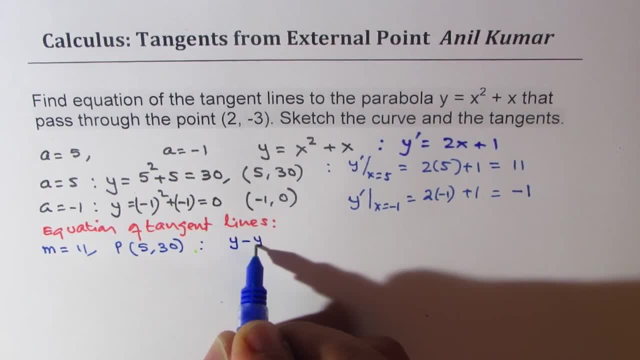 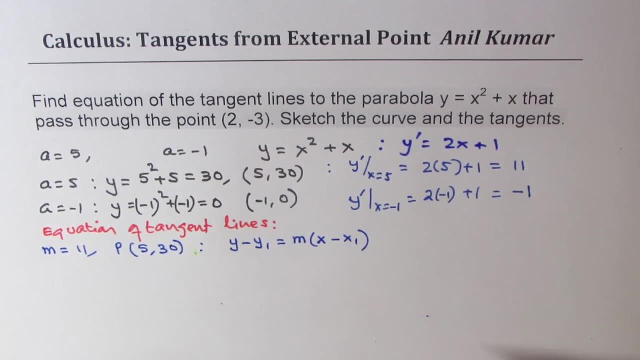 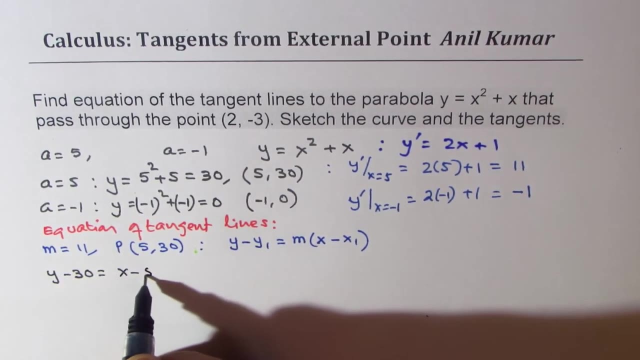 We'll use the equation of the line of the form: y minus y1 equals to m times x minus x1.. So using this, we can find our first equation, which will be: y minus 30 equals to x minus 5 times slope of 11.. 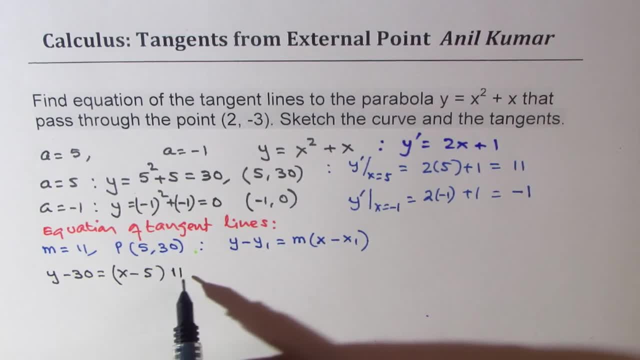 Let me write here now. Okay, So we'll open this bracket. So we get: y minus 30 equals to 11x minus 55.. Bringing all the terms together, we get our equation as- let me push this page a bit- 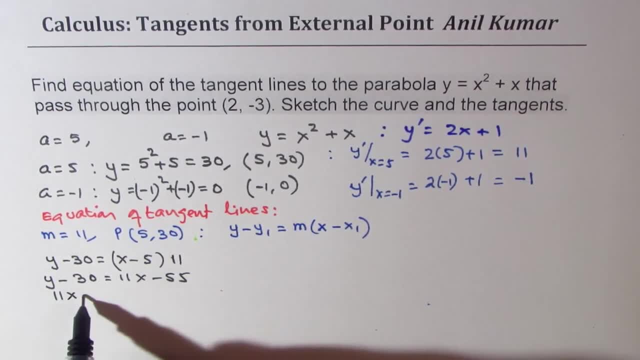 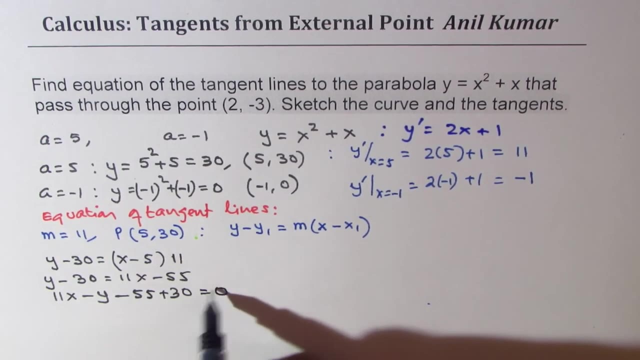 Okay, So we get 11x minus y And we have minus, so this gets added up. So let me write here: minus 55 plus 30, right? So that is the first equation- equals to 0.. 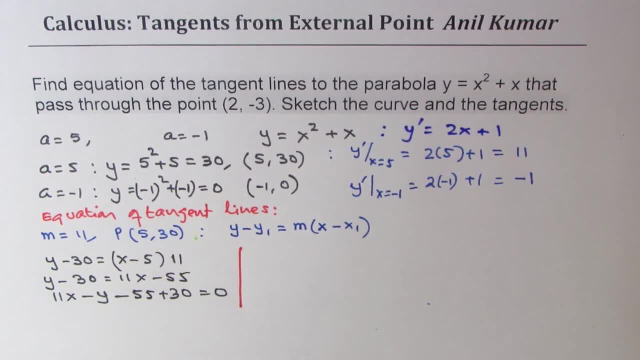 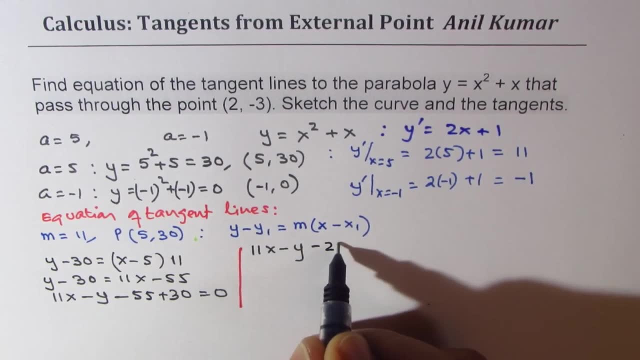 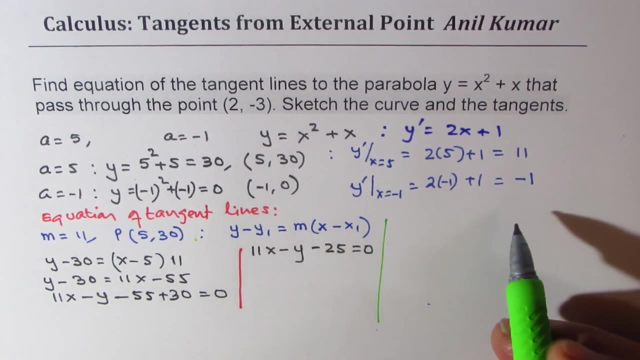 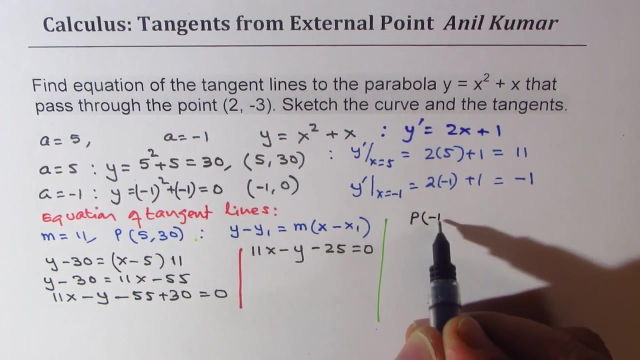 So let's rewrite this as 11x minus y, And that is minus 25 equals to 0.. So that is our first equation. For the second equation, we'll use the point with slope minus 1.. So the second equation, the point given to us is minus 1, 0.. 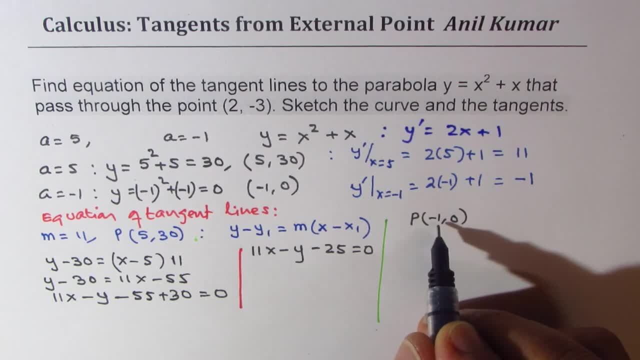 So that's the y-intercept. Okay, That's the x-intercept minus 1, 0.. And the slope m is minus 1.. So we get y minus 0 equals to slope of minus 1.. So let's say: minus times x minus minus 1.. 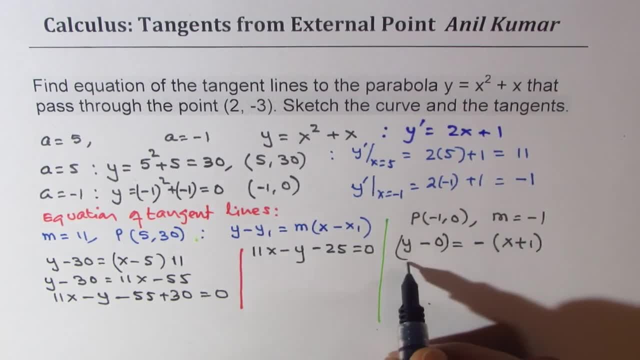 So x plus 1.. So we can open this bracket. So we have y equals to minus x minus 1.. Bringing all the terms together, we get x plus y plus 1 equals to 0. So these are the two equations. 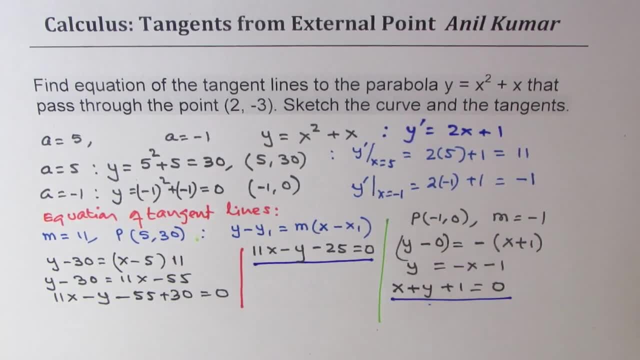 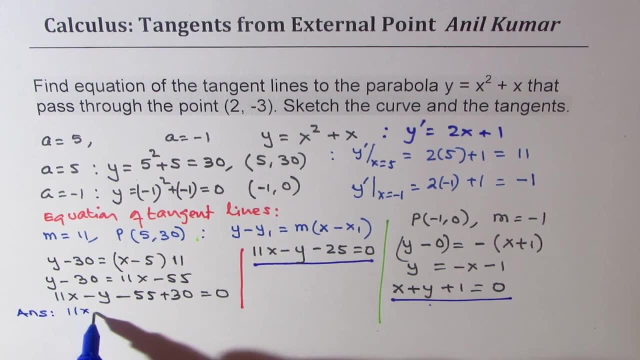 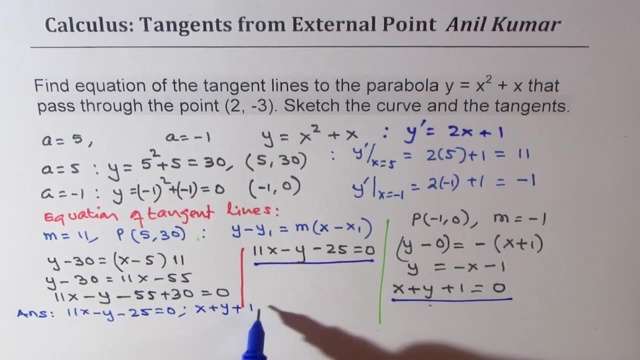 So now we can write down our answer. The equations are: 11x minus y minus 25 equals to 0.. And the second one is: x plus y plus 1 equals to 0.. Let us sketch in the previous page. 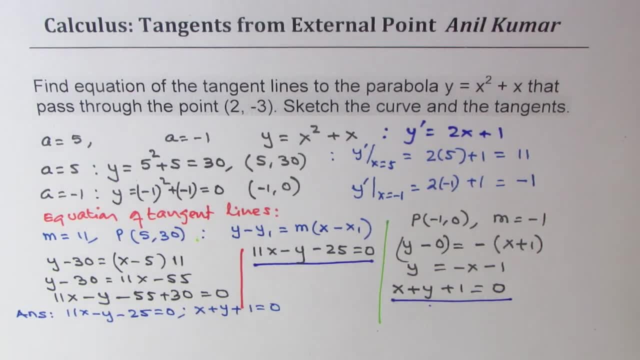 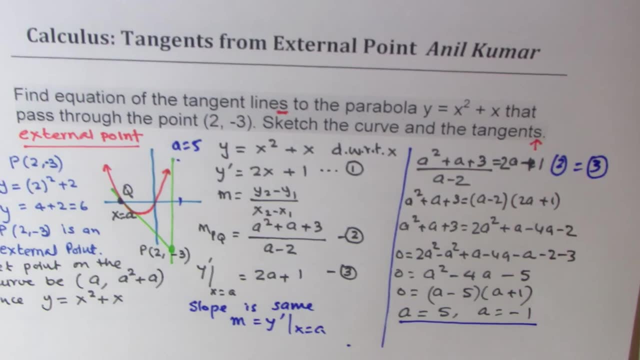 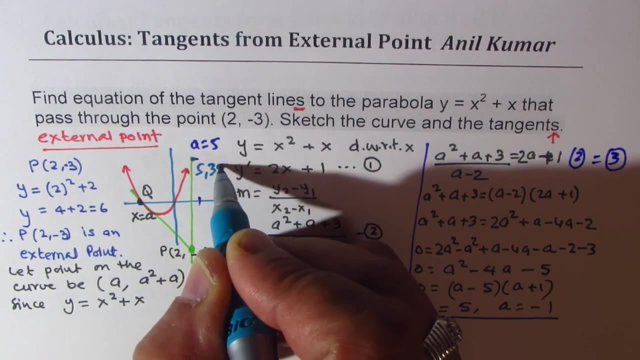 Or let me share that page with you now. Okay, So the second point here is for the value of 5.. We have 30.. Anyway, So here is our sketch. You can make a better sketch. So somewhere there we'll have a point which is 5, 30.. 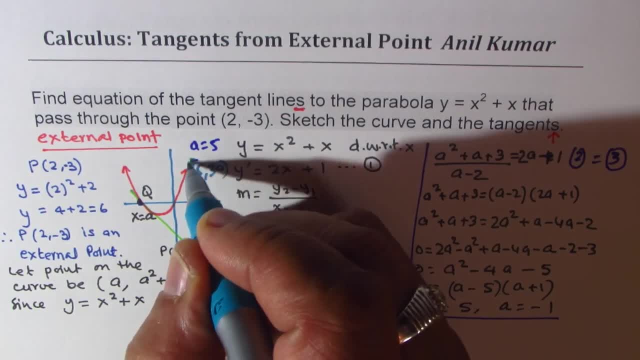 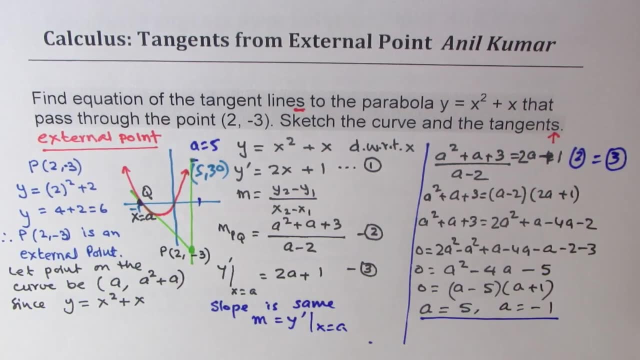 And this is the point 2, 3, that forms the. you know, when you extend it, And this is the x-intercept at minus 1.. Correct, You could always write this equation as: y equals to x is common.